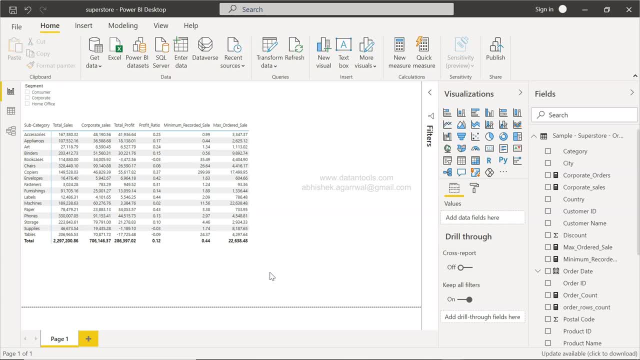 is for the google data studio report, which contains all 900 plus videos related to various different topics, like the click view, click sense, power. the power bi is already part of this um tab, blue python- all of those are present over there and you can quickly search there. all right, so now. 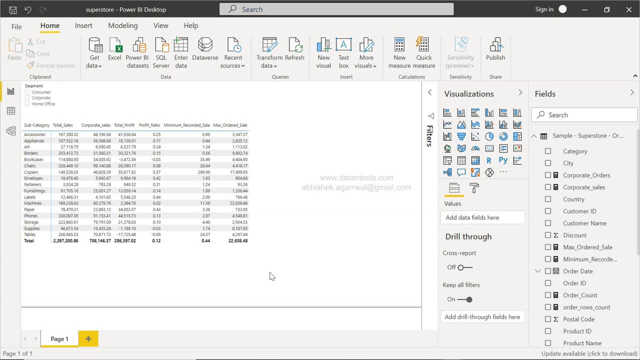 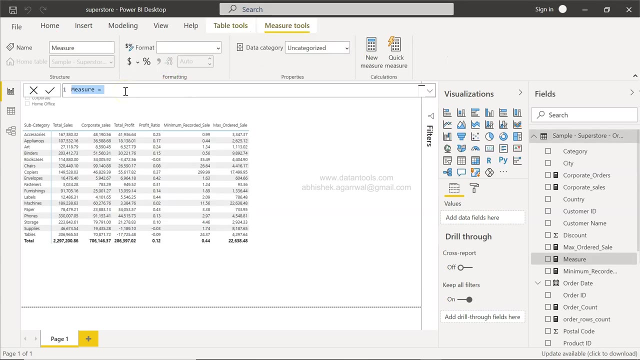 with that information, let's move ahead and create the average sales for our metric. all right, to do that, what we need to do is click on the new measure, and once we click on the new measure, it will give us the formula bar and we will going to write the name of the measure, which is the average. 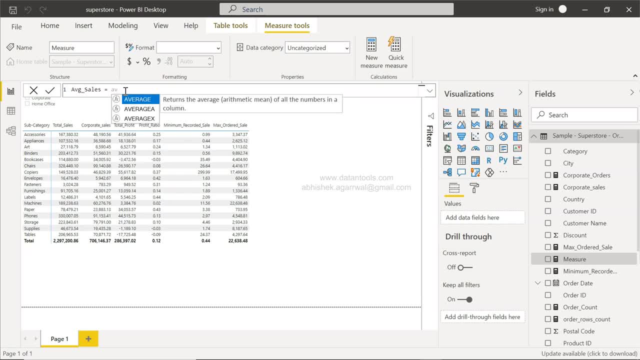 sales and we will use this function, which is average. once we have average, then we will provide the sales as the field or whatever field of our interest and close the parenthesis the minimum number of setting or the minimum setting that you need to do to find the average. 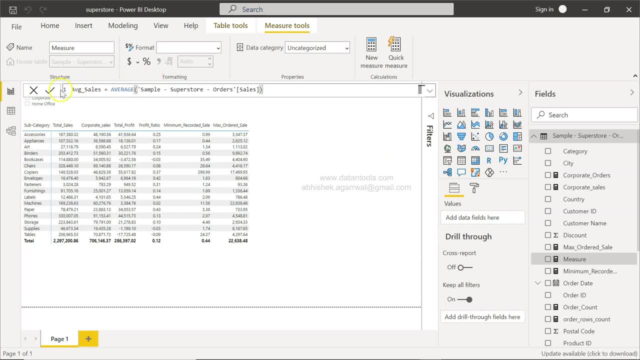 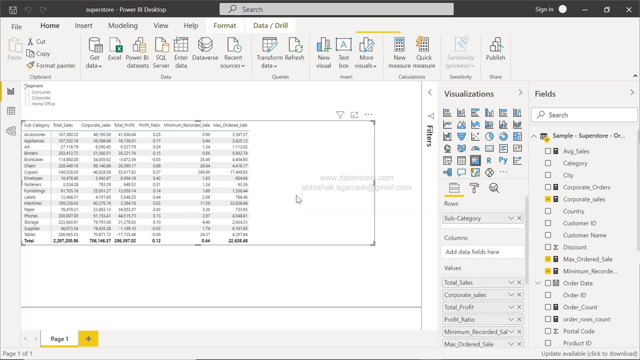 sales for your metrics. all right, once you are done, you click on this, sign over here and the field will be created with the name average sales and it is present over here, right, to add this to this table. we will click on this table over here, right, and come over here on the average sales and drag it to. 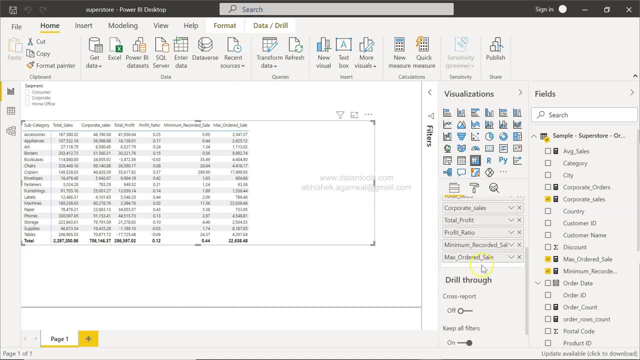 values. so i will just scroll this up. so the last value is present and i will put it right after the last value. all right, so here we have the average sales coming as the value, with two decimal points. we can format it if you want it. but mainly what i want to show you, 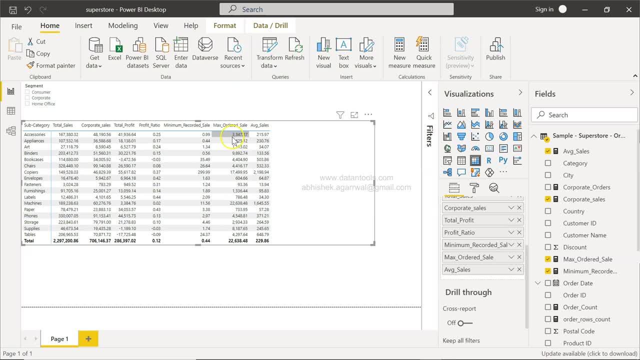 is how the average sales is coming. so over here you have maximum order sales, you have average sales, you have minimum recorded sale. this is the total sales that you are having, so gives you some sort of a ballpark idea, as the range is quite high, from lower value to higher value to the average value. 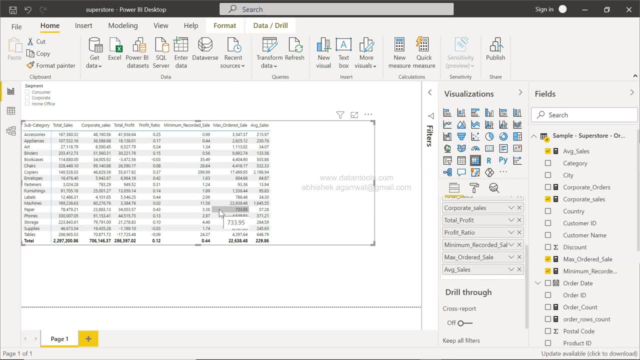 and gives, gives us an impression as to a lot of activity is going on and because of which the, the ranges are pretty high. but all in all, you get to know what is your average sales for these categories and very quickly, i have. i will just show you in case if you need to remove the decimals, because it does not make. 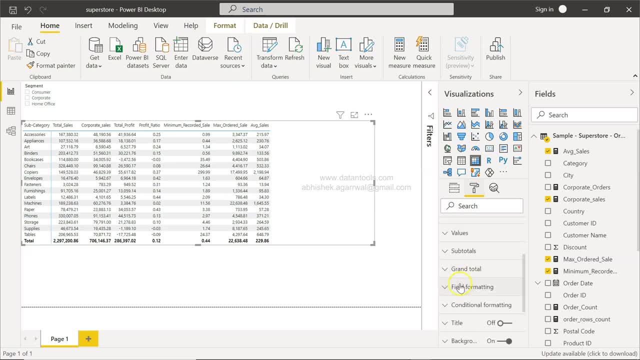 a whole lot of sense. then what you can do is you can come first of all to this formatting, then field formatting, and then choose the field which you want to format, like average sales over here, and for value decimal points instead of auto, you use zero and the decimal points are gone. all right, 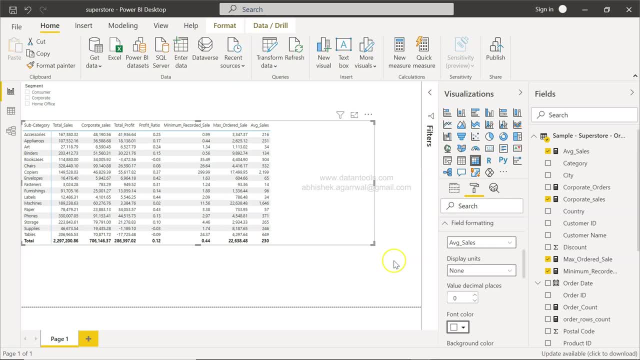 that's what you need to do, and i wanted to show you, uh, finally, what, uh how you can format these fields, and that's about it. i'll meet you now in the new video with the new topic.